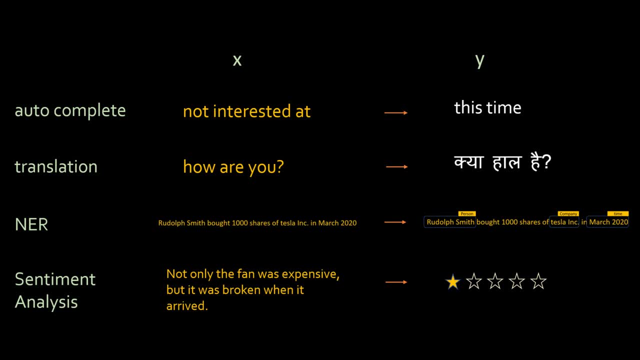 where using sequence models or RNN- recurrent neural network- helps. The fourth use case is analysis, where you have a paragraph and it will tell you the sentiment, whether this product review is one star, two star and so on. Now you would think, why can't we use a simple neural? 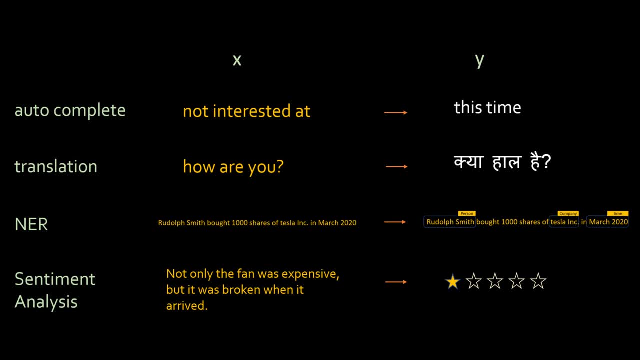 network to solve this problem. See all these problems. they are called sequence modeling problem because the sequence is important. When it comes to human language, sequence is very important, For example, when you say how are you versus you or how doesn't make sense, right. So the sequence is important here. And you would think 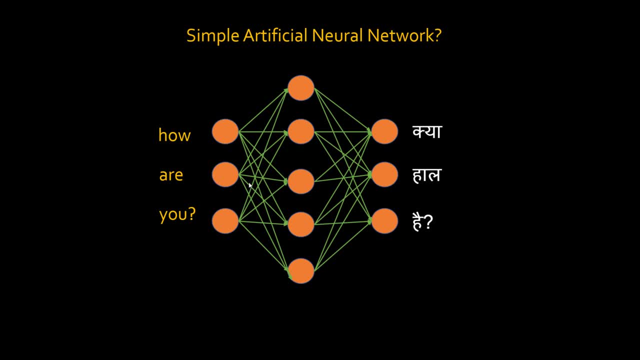 why don't we use simple neural network for that? Well, let's try it. So for language translation, how about we build this kind of neural network? you know where input is the English statement and output could be in the statement. Once I build this network, what if my sentence size changes? So 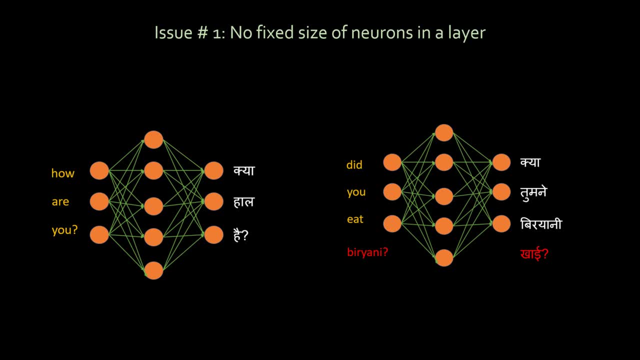 I might be inputting different sentence size and with a fixed neural network architecture it's not going to work because you have to decide how many neurons are there in the input and output layer. So with language translation number of neurons becomes a problem Like which: what do? 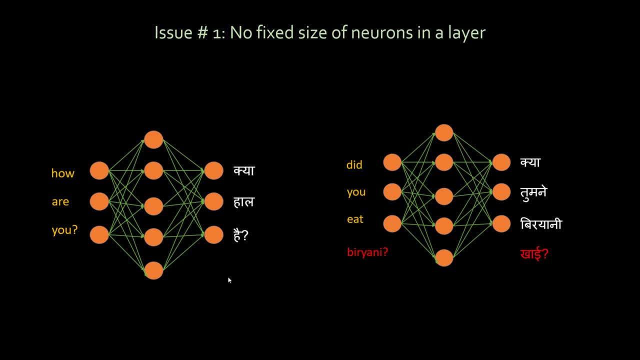 you decide as a size of neurons. Now one would argue: okay, I would decide, let's say a huge size, let's say 100, 100 neurons and remaining if I'm saying: did you eat biryani? so it will. 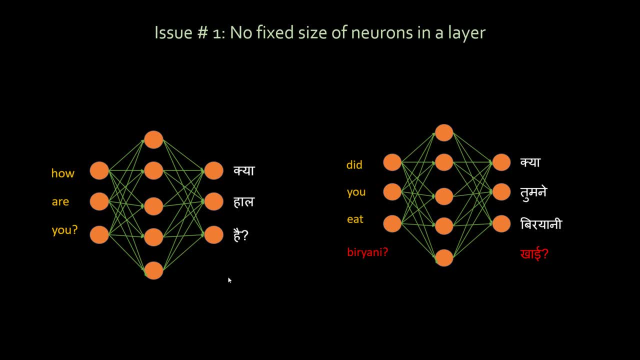 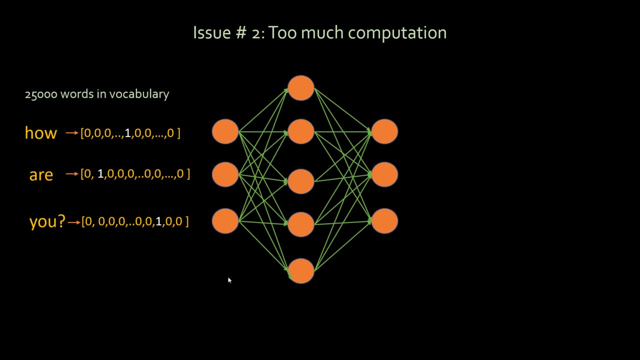 be four neuron, remaining 96, I will just say zero or you know, blank statement. That might work, but still it's not ideal. The second issue is too much computation. When you all know neural networks work on numbers, they don't work on string. So you have to convert your word into a vector. So one of 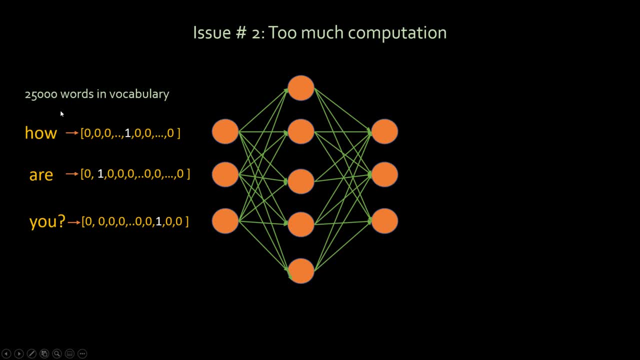 the ways of converting that into a vector is: let's say, there are 25,000 words in your vocabulary. you will do one hot encoding where you know how. let's say is: at 46 position R is, let's say: 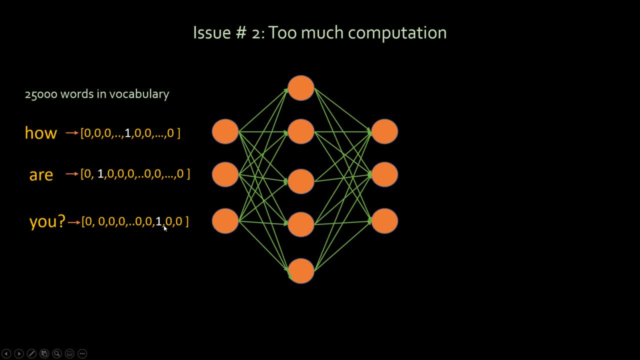 at second position U is, let's say, at 17,000 position. So at that position you put one. remaining position you put zero, and that's called one hot encoding. You have to do similar thing for output as well, but you realize this will increase too much computation. Each of the 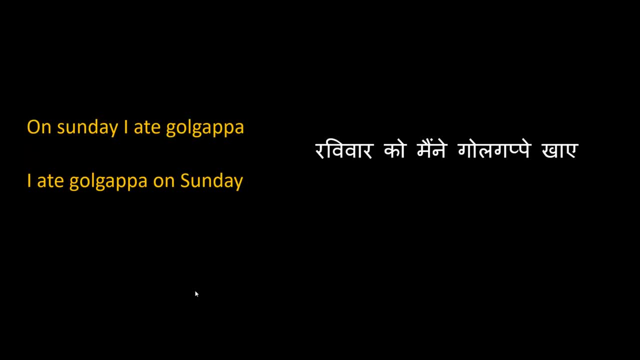 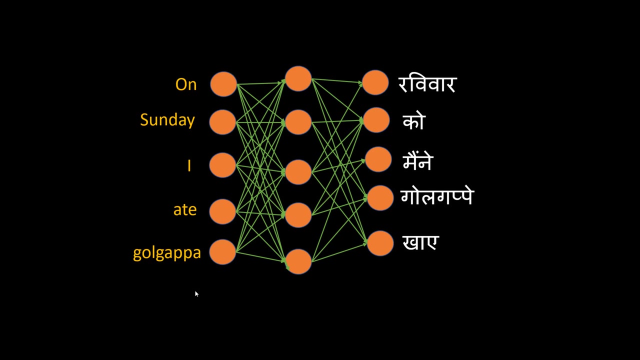 output layer itself is humongous. The third issue is this: Sometimes, when you translate language, you for, let's say, two different English statements, you might have a single Hindi statement. So in this case, when I say on Sunday I ate golgappa, let's say I trained this network. 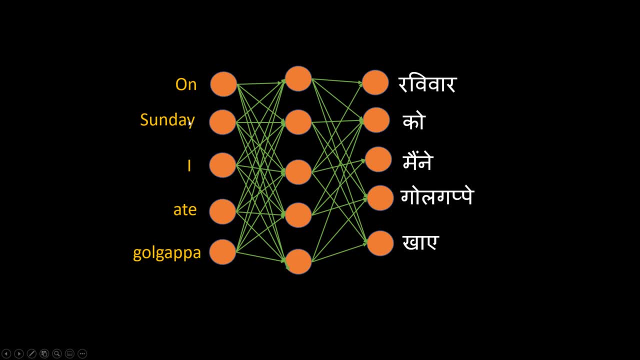 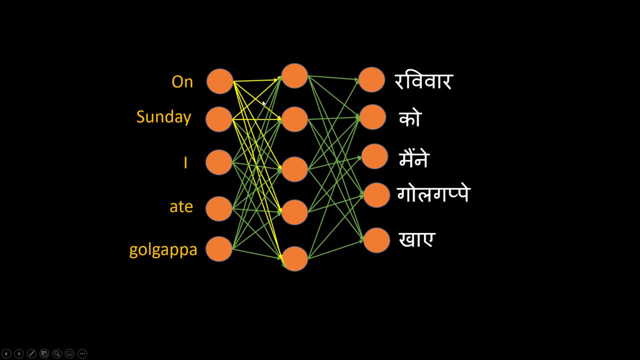 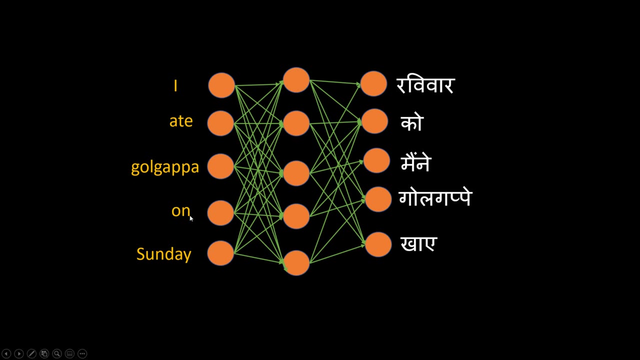 based on this statement. And then for on Sunday, let's say it will adjust the weights of all these edges which I have highlighted in yellow color. Same statement I can say differently. I can say: I ate golgappa on Sunday. So now, on Sunday, the meaning of on Sunday is same, but here neural. 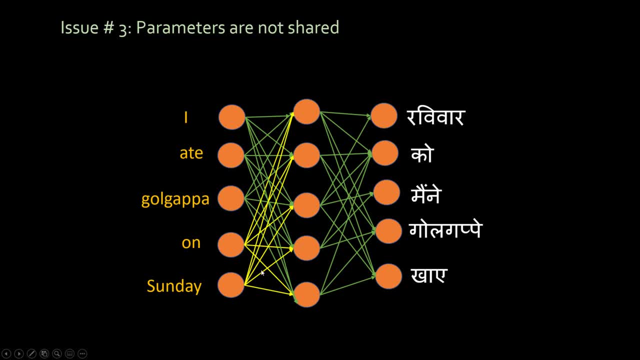 network has to learn different set of edges. You see, all these edges are in yellow color, So the parameters are not shared. We looked at in our convolutional neural network tutorial as well that by using convolution operation we can share the parameters. Here the use of ANN or artificial neural network doesn't allow you to do that. 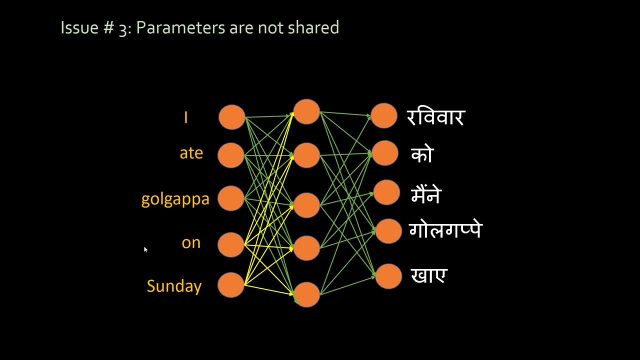 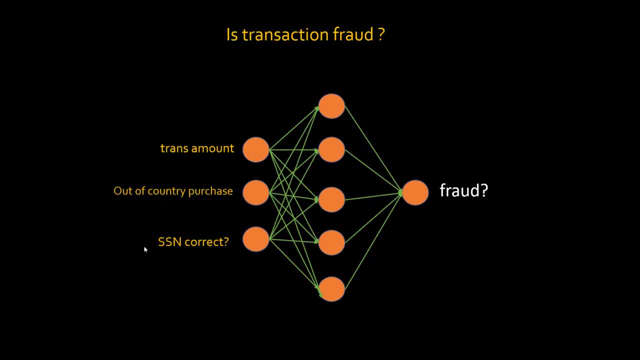 Okay, Also, the most important part in all this discussion is the sequence. See, when you have structured data, for example, you're trying to figure out if the transaction is fraud or not. And let's say, your features are transaction amount, whether the transaction was made out. 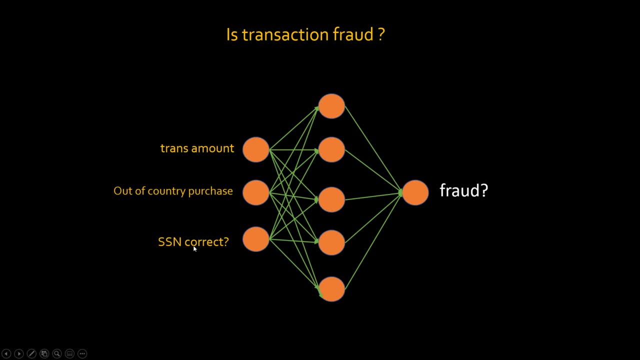 of country, or whether the SSN that the customer provided is correct or not. Now here, if you change the order of these features, let's see. the SSN is correct. I supply in Of my first neuron. it's not going to affect anything, you know. 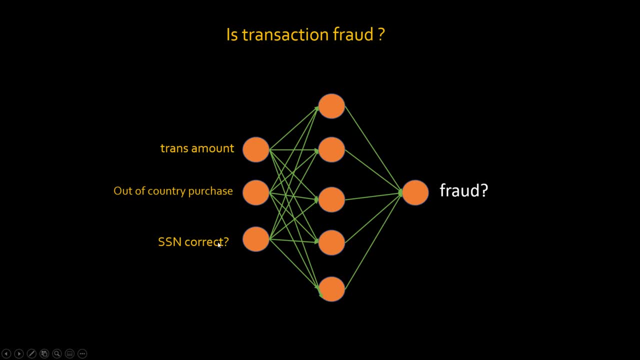 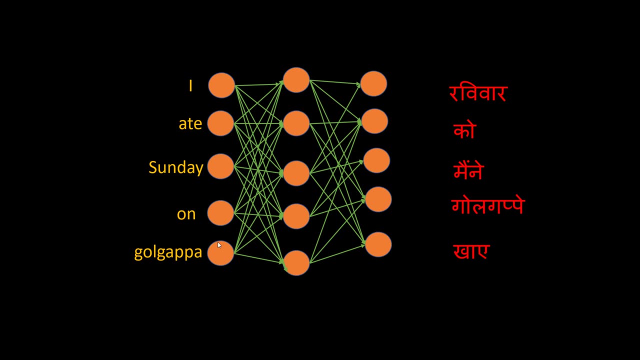 because the sequence in which you supply the input doesn't matter, Whereas if you have English, pange English to Hindi translator translation. and instead of saying I ate Golgappa on Sunday, when I say I ate Sunday on Golgappa, 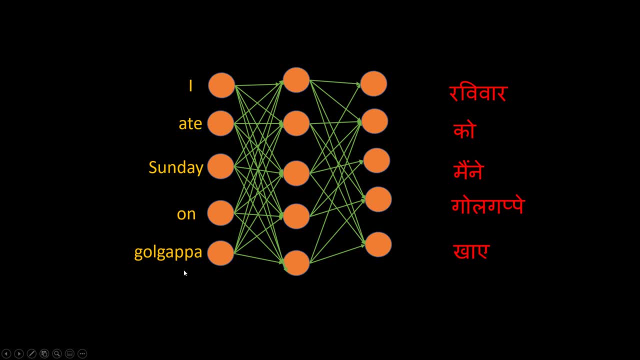 And if I say I ate Sunday on Golgappa at sunday on golgappa, the meaning becomes totally different. so now you cannot say that the hindi translation is ravi arko maine golgappa khai, because it becomes invalid. so sequence is: 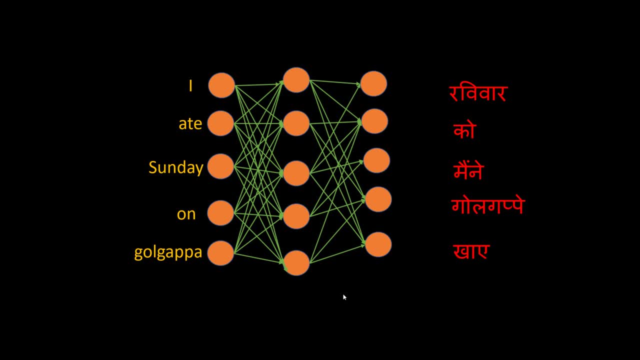 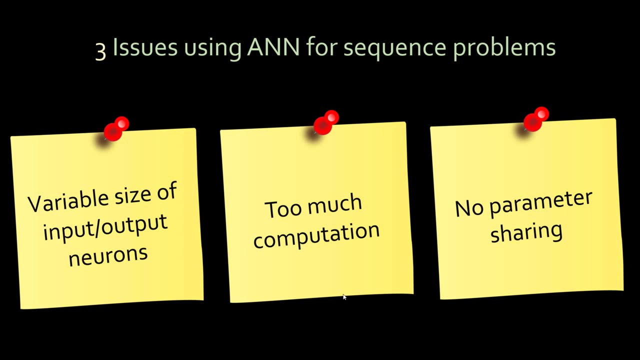 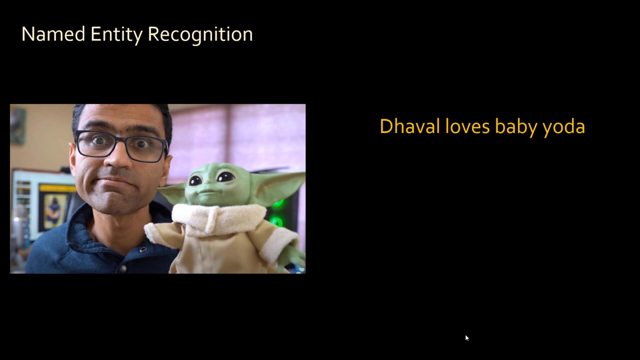 very, very important. that's why artificial neural network doesn't work in this case. just to summarize, these are the three major problems with using ANN for sequence problems. let's once again talk about name entity recognition. let's say: the world loves baby yoda, i love my baby grogu, i love mandalorian series and we have got this nice baby grogu at our home. 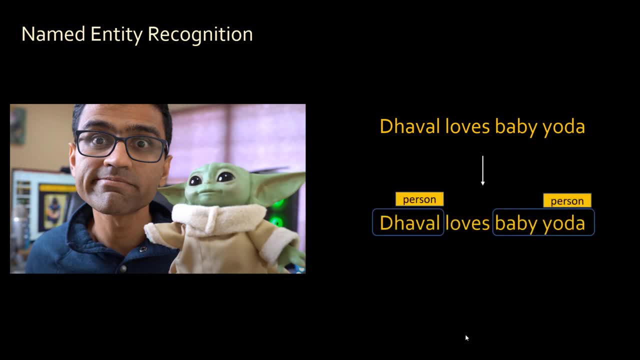 which actually talks with us in this statement. the world and baby yoda are person names. okay, so the whole purpose of name entity recognition is to find the name of the baby yoda and to find the name of the baby yoda, find out the entity you know like double as an entity, is a person. baby yoda as an entity, as a person. 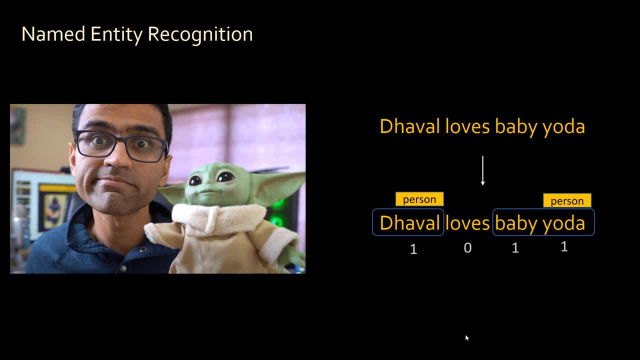 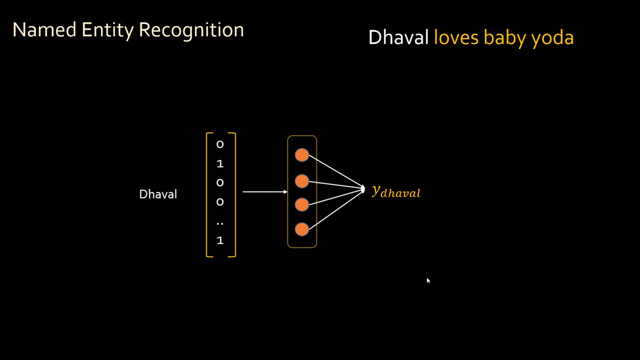 so that's the whole goal of any r. now you can represent this as ones and zero. so if the word is person name, you would mark it as one, and if it is not person name, you mark it as zero. so let's see how RNN works here. RNN is also called recurrent neural network. 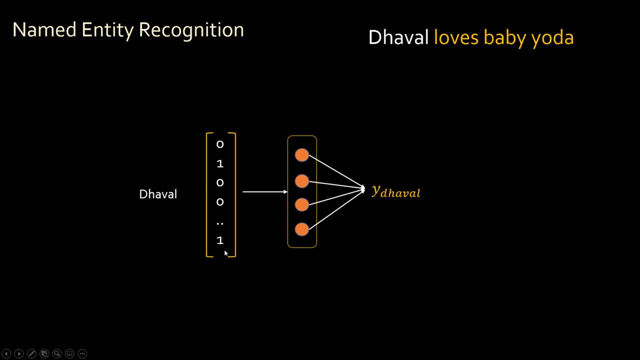 so first of all you have to convert the word into some vector. doesn't matter how you convert it. you can take a vocabulary and use one hot encoder, and there are other ways of vectorizing a word. then you have a layer of neurons, so these are all individual neurons. let's say this is one layer, it's a hidden. 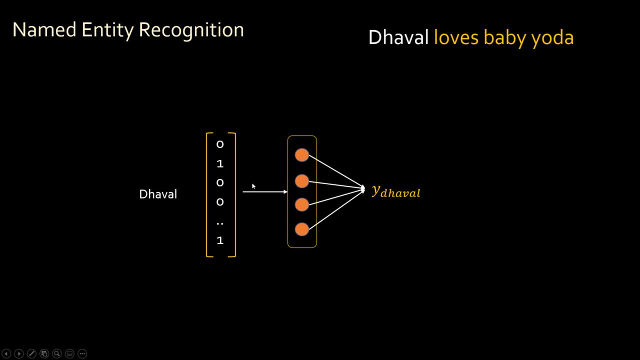 layer, you supply that and you get one output. okay, so each neuron, all you know, has a sigma function and a empty say особy be. all you know, here's a sigma function and every altre so and so. level of forward singular mass, which is zero, equals prank. okay, so each neuron, all you know, has a sigma function. and add, which will 모르, various cos�� 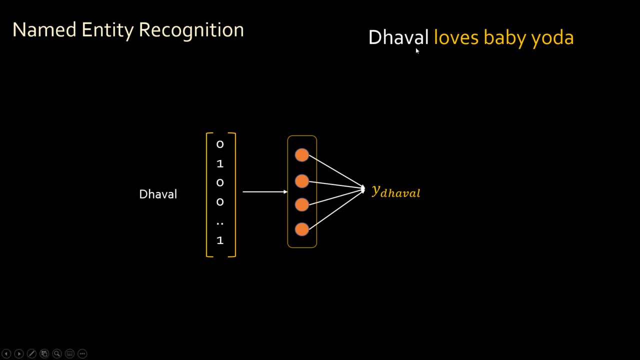 activation function. So now, while processing the statement the world loves baby Yoda. now I will process it word by word. So I supply the world, get the output and then I go back again. Now I supply loves, convert it in vector and the previous output which I got, which was y- the world. 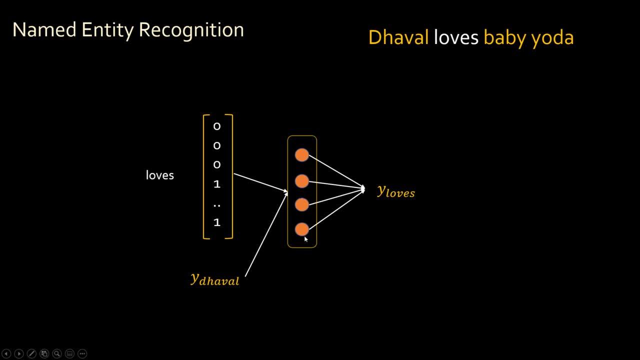 INS supply that as an input to this layer. So you see, the input of the layer is not only the next word but the previous output, Because the language makes sense. language needs to carry the context. If I just a word loves and if I don't have the world in front of it, it it might mean a different thing. 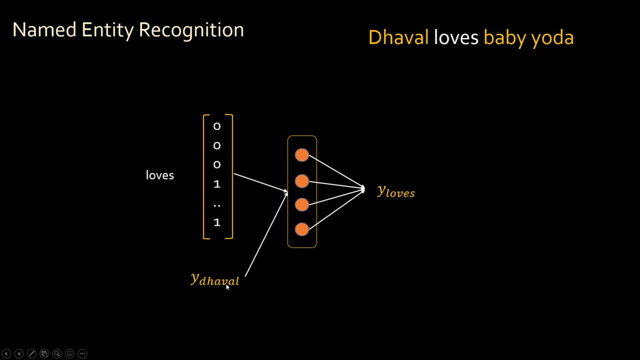 So there is a context that you need and this kind of architecture provides you a context or a memory. In the third word, again, you supply baby to the same network, right? So our network has only one layer. It has only one layer. So there is input layer, output layer and the hidden layer is just one and it has a bunch of neurons. 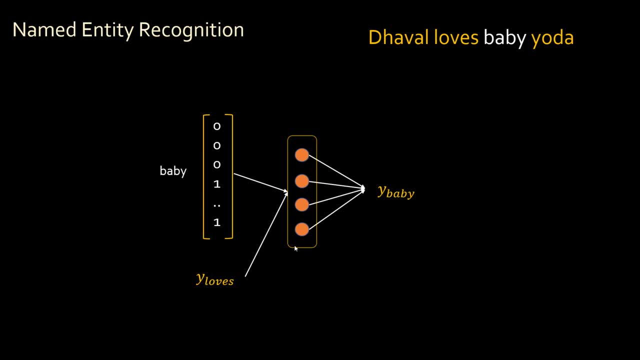 In that we are repeatedly processing word, one by one, okay, And you keep on doing this. Now, the benefit of this is when I'm processing baby, when I get y loves, that y loves carries the state, the previous state or previous memory of. 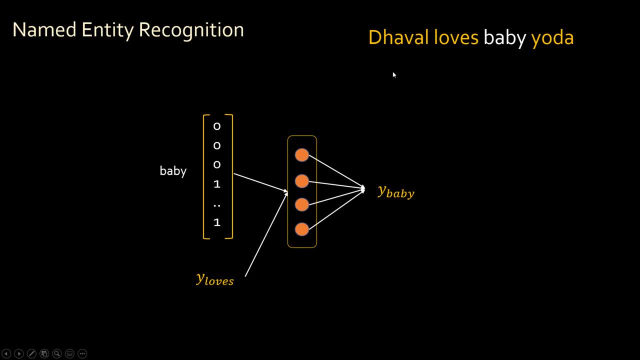 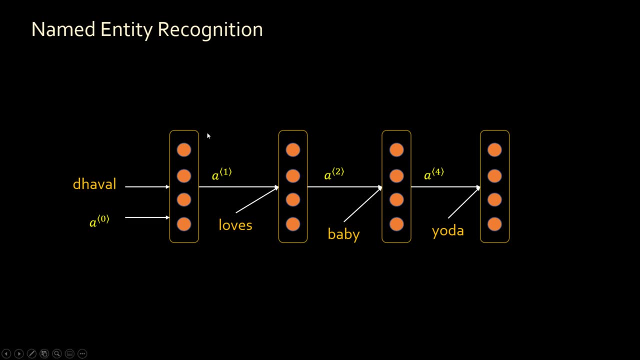 double loves. you know The whole statement. Now I'm presenting this in a different way. Make sure these are not four different hidden layers. This is a time travel. okay, So actual hidden layer is only one. I am just doing a time travel. 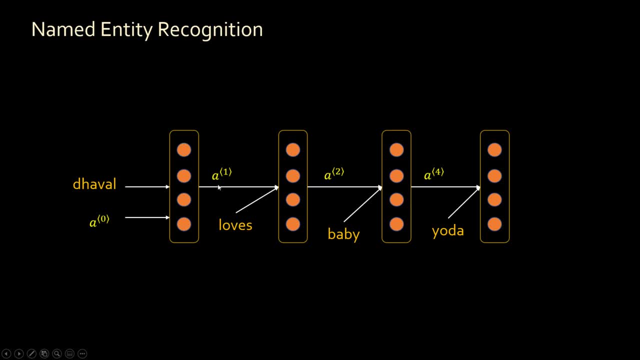 So first, when I supplied world to the world, I got this output, and output was nothing but the activation function which I am denoting with a1, and you need some previous activation, a 0 as well. Let's say it's a vector of all zeros. 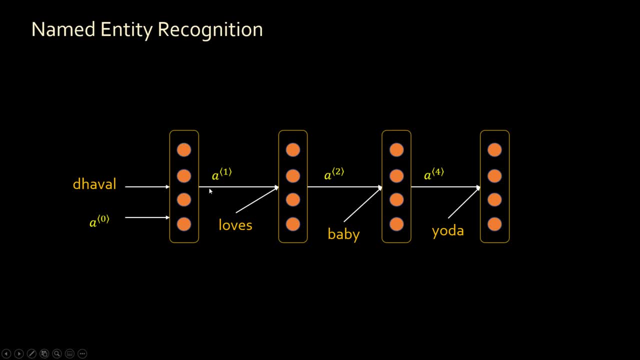 then you supply a second world laws and use the previous output, which was wide double. So wide double and A1, they're both the same here- and then you get another output, A, two, where that is supply along with the third word, baby- to the same. 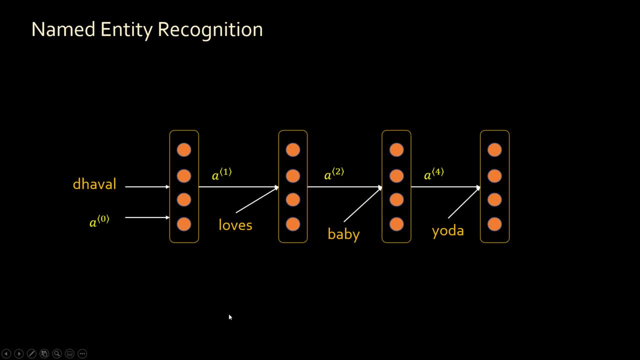 network. So this four neurons, it's the same single layer. I am just showing different the status of it at different times. okay, so you have to be very clear on this that these are not four different layers, it's just one layer, just because I am showing different time steps. that's why I'm 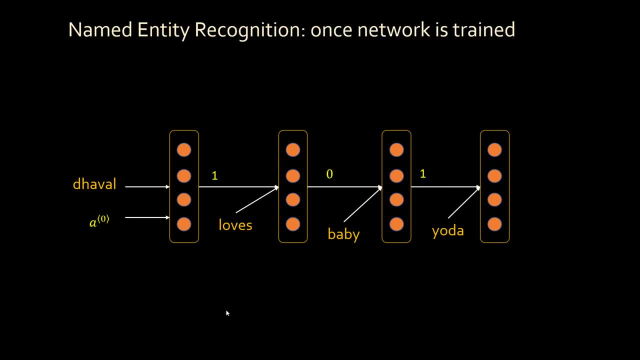 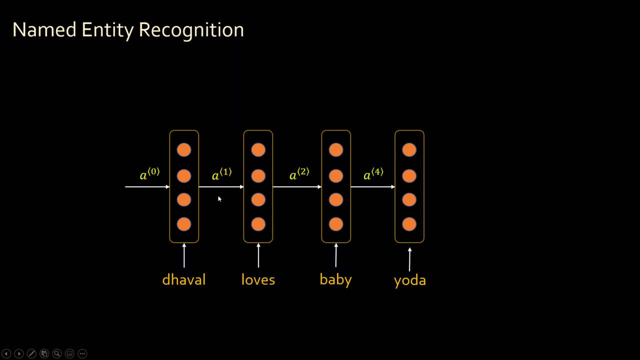 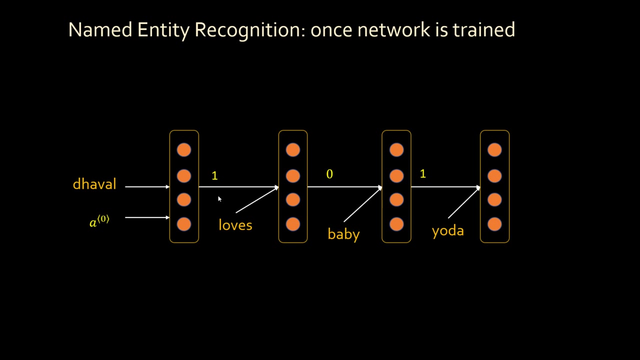 showing you almost a time travel here. and once the network is trained, of course it will output like double is one, loves is zero, baby is one, and so on. okay, so you get your NER output individually here, one other way of representing a same network. okay, because just to avoid confusion and to make presentation a 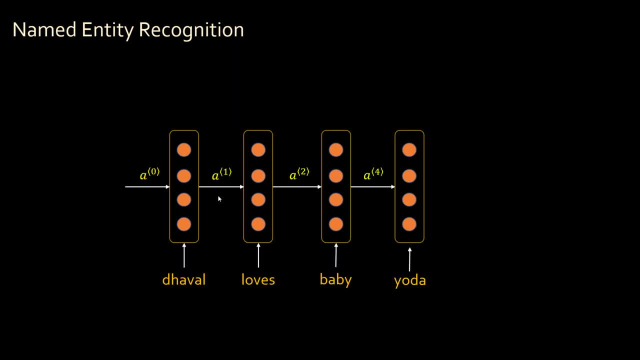 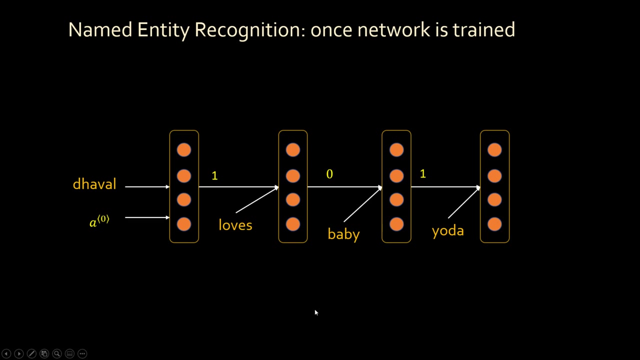 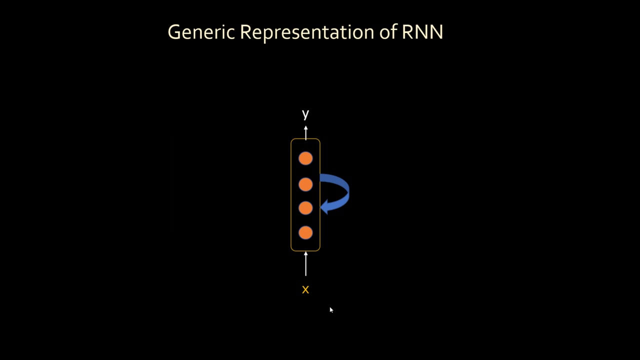 little more clear. many times in literature you will see presentation like this, where each word which is an input comes from the bottom and there is activation. so again, this and these two diagrams are exactly same. okay, I'm just putting this word at the bottom. generic representation of RNN is this. so this is the real. 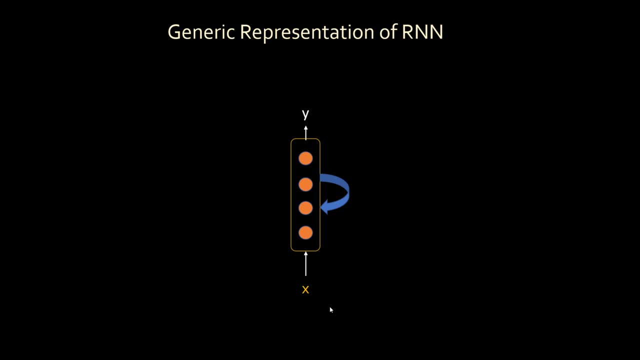 representation. you have only one layer and you are, you are kind of almost in a loop, you're- you're supplying the output of previous word as an input to the second word. so now let's talk about training. so again, the problem we are talking about is NER, where these are my training samples: okay, X and Y, X and. 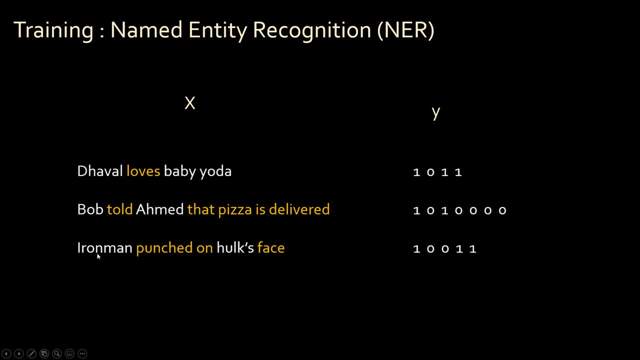 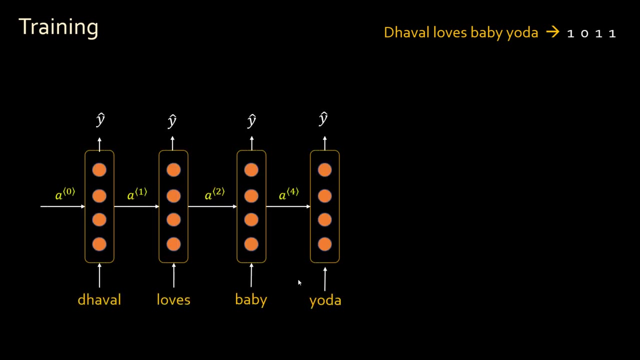 X is a statement, Y is whether a given word is person name or not. so we are processing first training sample. double loves, baby Yoda. so this one. I will first initialize my neural network weights with some random values, then I supply each word, then I calculate Y hat which is predicted Y, and you see. 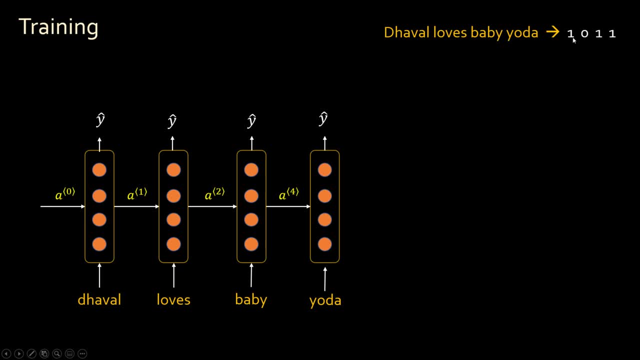 y, then i compare with the real y. so real y here is 1 0, 1, 1. so i compare that with here. so 1 0, 1, 1. i compare that with y hat and i find out the loss. okay and that, and then i i sum the loss. 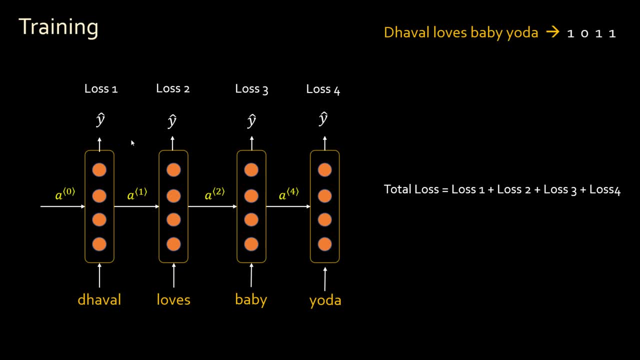 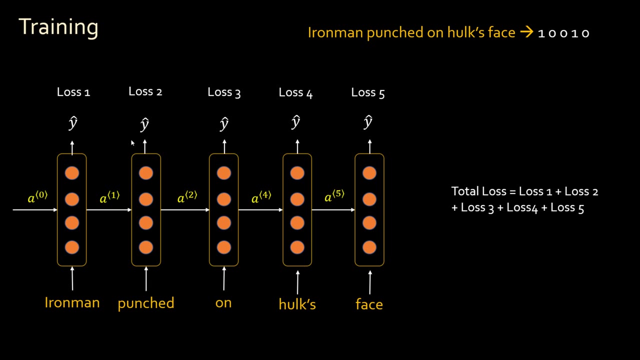 so that will be my total loss. you all know about gradient descent, right? so we compute the loss, then we back, propagate the loss and we adjust the weights. so now i take the second statement. iron man punched on hulk's face. he was very angry with hulk. again i calculate all the losses. 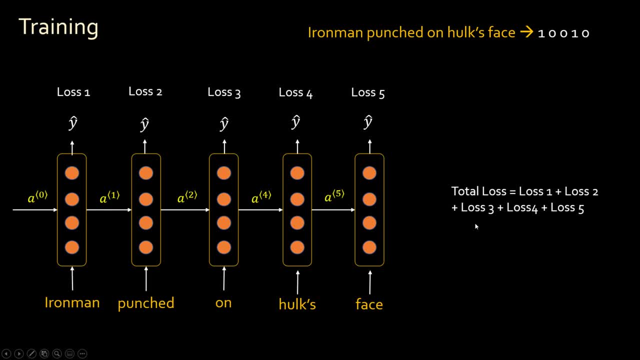 then i find total loss and then i do gradient descent to reduce the loss. so i keep on doing this for all my training sample. let's say i have a hundred training samples. passing all hundred training samples through this network will be one epoch. We might do, let's say, 20 epochs and at the end of 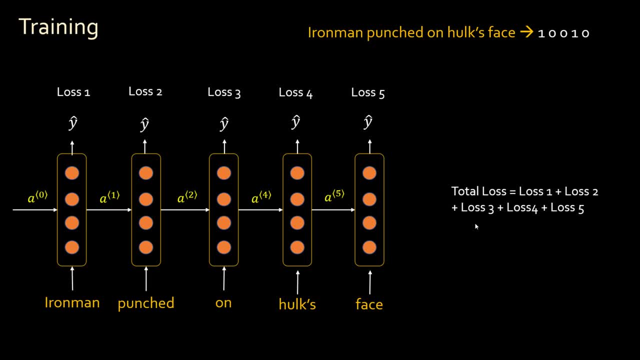 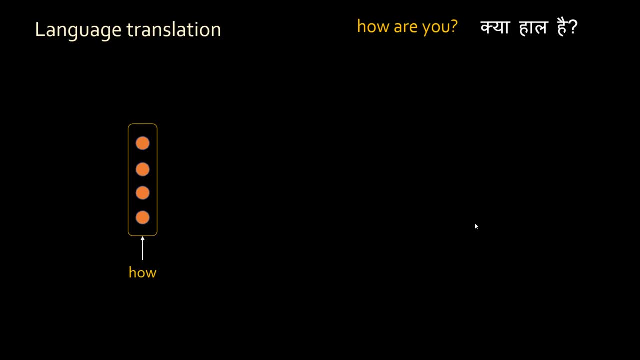 the 20 epoch, my loss might become very minimum. At that point we can say: my neural network is trained. Let's take a look at language translation. So in language translation what happens is you supply first word to your network, then you get the output, then again same network, you supply second word and the 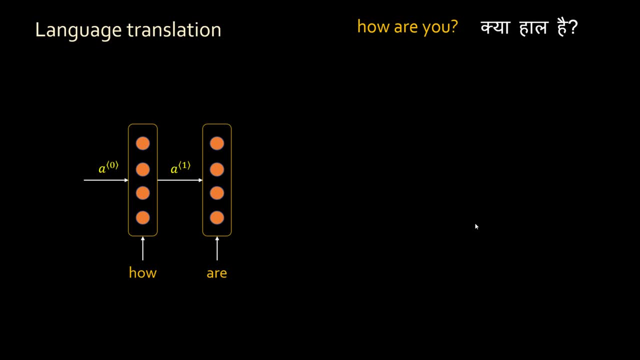 output from previous step as an input. and, of course, when you supply first word, you have to pass in some activation values, let's say all a vector of all zeros. then you supply third word, fourth word and so on, and when you're done with all the words, that's when the network starts to translate it, because 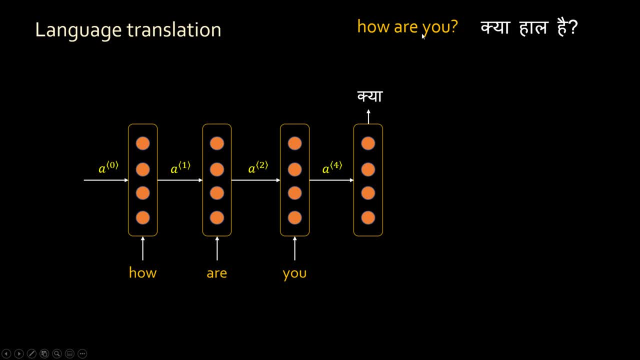 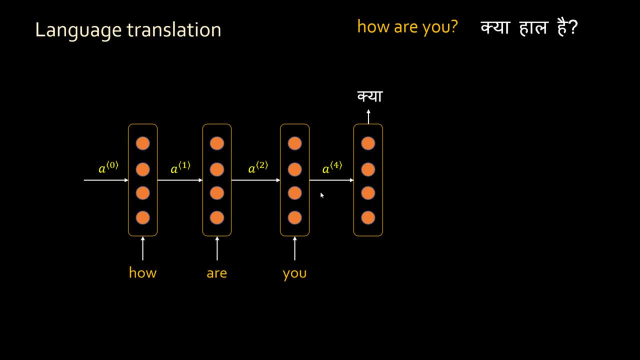 words and only then the network can translate for you. So the network will translate it like this: and the first part is called encoder, the second part is called decoder. We will go more in depth into all this, but I want to quickly demonstrate how the neural network looks. 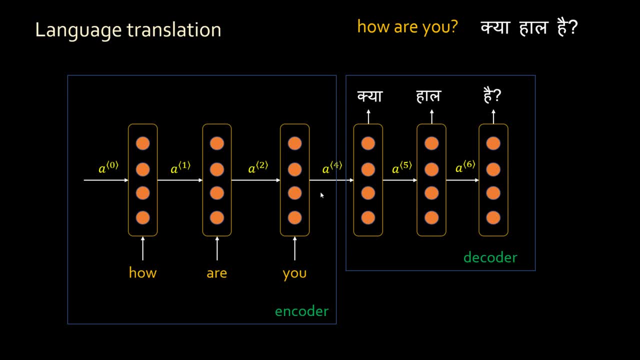 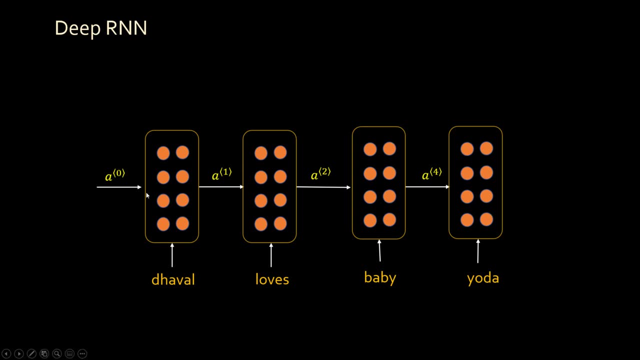 in the case of language translation. now, this layer doesn't have to be just single layer. it can be a deep RNN as well, where the actual network might have multiple hidden layers. okay, so I hope that clarifies the architecture behind RNN and you understand why you can't use simple neural network here and you have 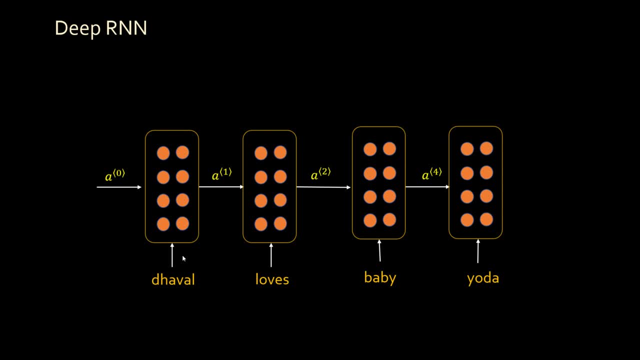 to use specialized neural network called RNN- and we'll talk about that later- which can memorize for you, which can remember previous state, because language is all about sequence. if you change the sequence, the meaning changes. so if you like this video, please give it a thumbs up and we'll be having more recurrent.